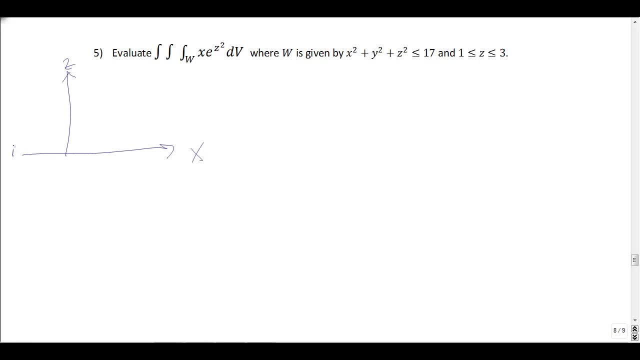 r in cylindrical being a radius, or maybe even zy. So we have some kind of circle That's radius, square root, 17,. and then these other bounds. z goes between 1 and 3, these are planes. So here's z equals 1,. do another one in red: here z equals 3, and so we're looking at this region. 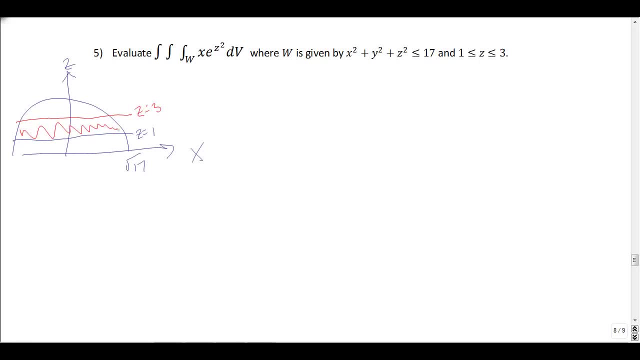 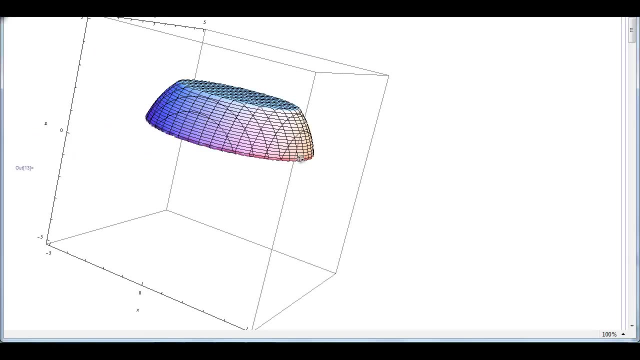 between those and that's rotated around here. So it's going to be some kind of almost disc-shaped thing here with a little bit of a curved side. So in Mathematica we can get a sense of what this looks like more precisely. So here's our three-dimensional image here. So this bottom is. 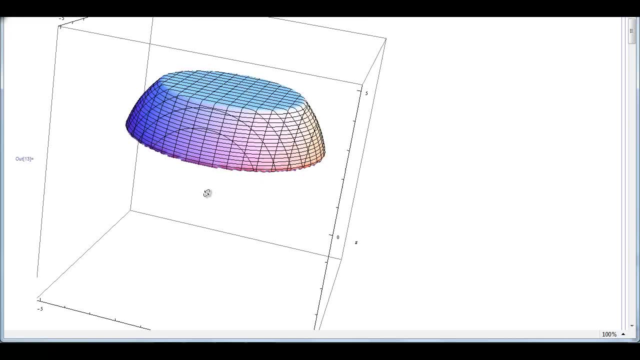 z equals 1,, top is z equals 3, and then we have a sphere where we're sort of just looking at the sphere, So we can just cut that down here. So this is really the shape we get. You could continue this. 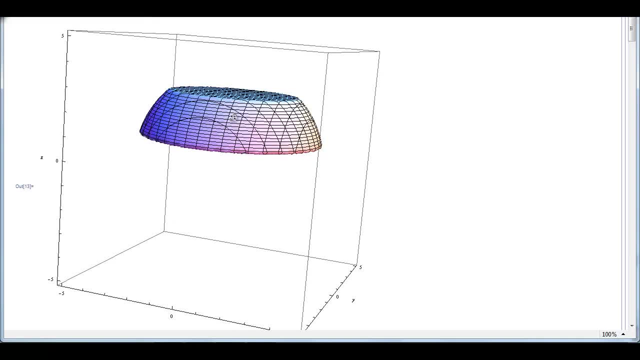 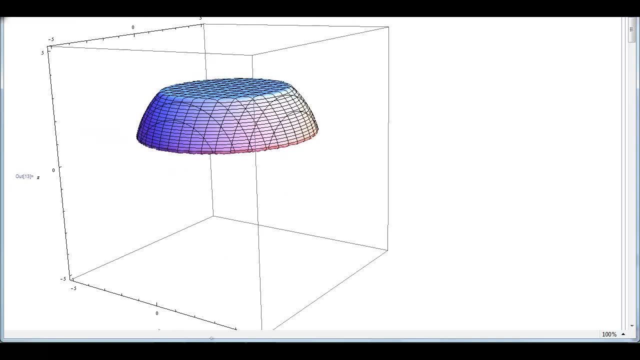 on to a sphere up, sort of finish the dome and then go below. We get this sort of- I don't know- bowl-looking thing maybe here. Okay, so that's the region we're integrating over Now, this region you. 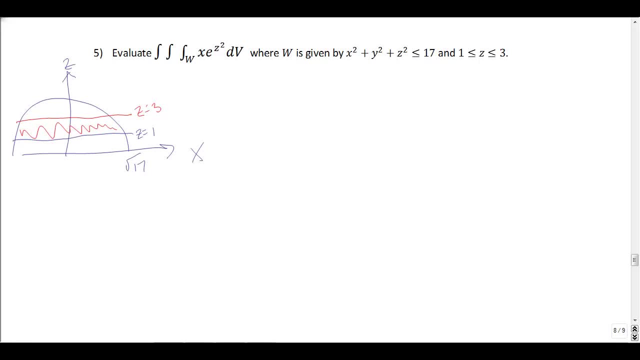 could integrate in spherical or cylindrical coordinates. We'll do both of those. They each are going to end up using two triple integrals. but this is an example of a problem where you can do this without sort of evaluating an integral at all. And the trick here is, if you notice, you have this x here, So the 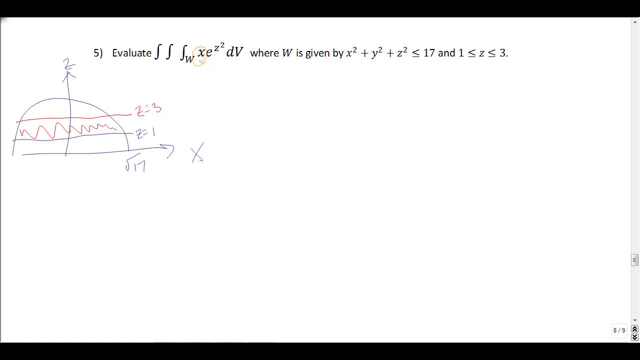 function you're integrating is an x. Well, x times e to the z squared. So that's odd in terms of x. So what that means is that if your region is symmetric about the plane, x equals 0, that's the yz plane. 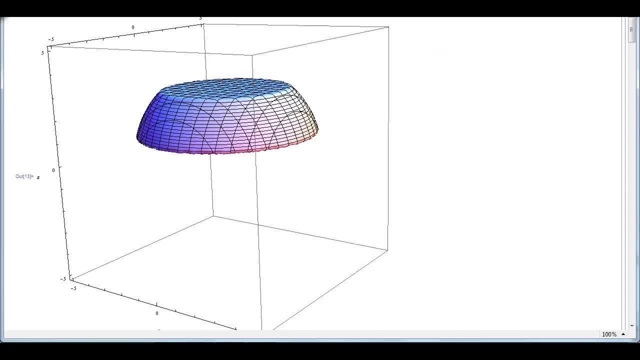 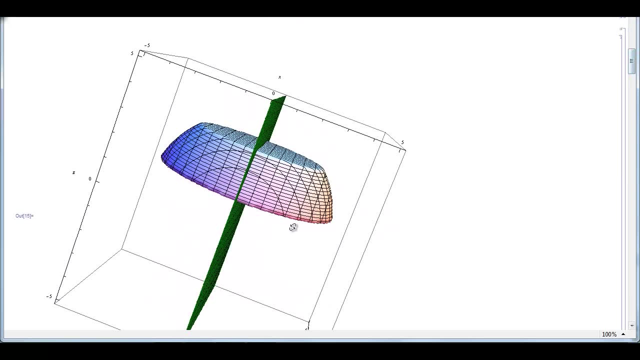 then your integral is going to be 0. And that's exactly what's going to happen. So when we look down here, here's this green plane- is the plane x equals 0, or the yz plane, And we get sort of the same sort of image with positive x's on the right and negative x's on the left. 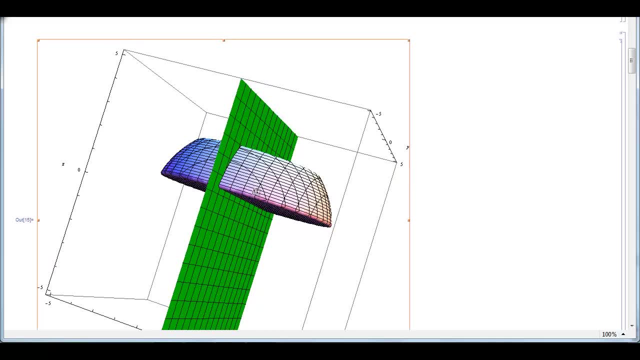 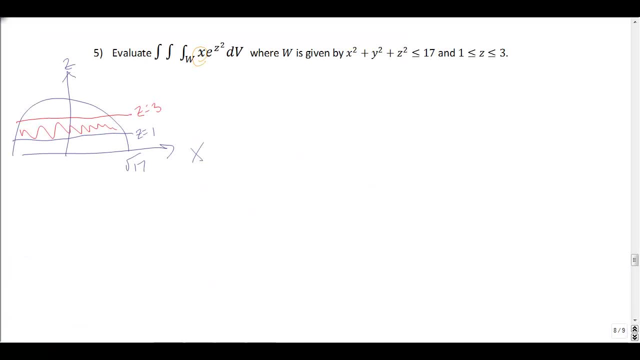 So what we can think about is: this is odd in x, and so if we integrate with respect to x first, that integral will be 0, whatever we have for bounds, and the whole integral will end up to be 0.. So, right away, 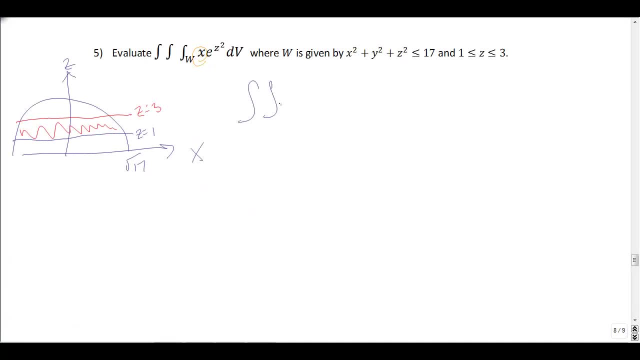 what I get, sort of a shortcut. I can get triple integral over w, x, e to the z squared, dv equals 0, and this is really by symmetry of w sort of about the maybe yz plane here. or we could say: x equals 0 here, Symmetry of w and yz plane. 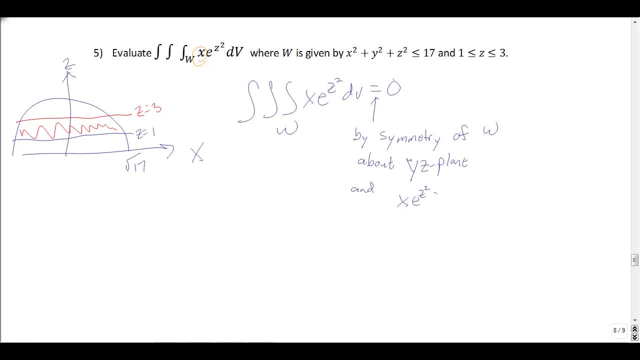 and x e to the z squared is odd really, if I just sort of view that in the x variable. So in some sense we get the 0 that way. Okay, So quick and easy. that's how you probably really ought to do this question. but we can kind of go through the exercise for the sake of just to set up the cylindrical coordinates and spherical coordinates for this kind of shape. 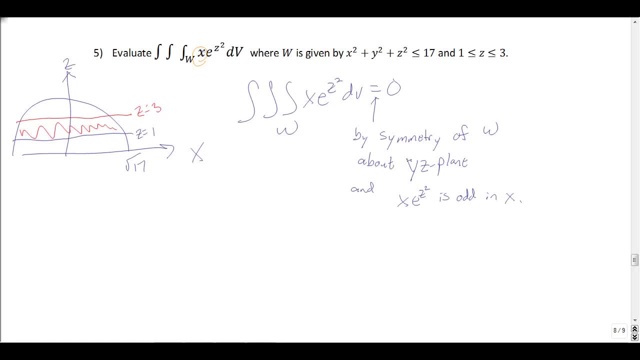 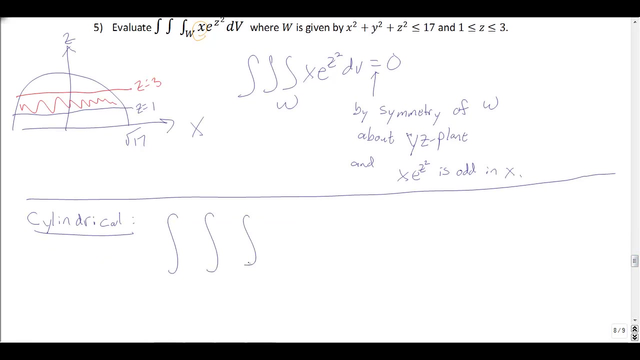 Imagine you didn't have an x there, you had something else. So I'm going to use the technique anyway. So let's do how about cylindrical first? So I'm going to do cylindrical coordinates, and so my integral. I'm going to get a triple integral of x. 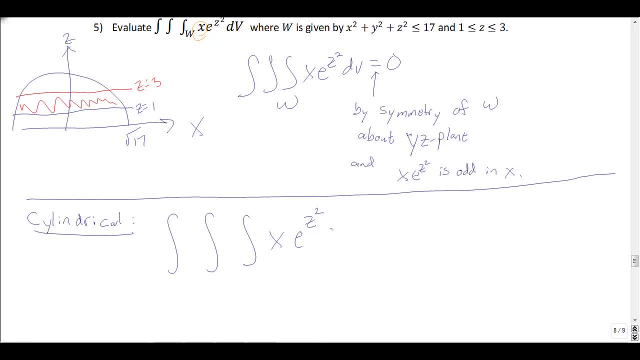 e to the z squared, except I should switch that to cylindrical. so the x, that would be r cosine, theta e, z is just z, and then I pick up an r for my Jacobian with cylindrical. Now I need to set up my bounds or my order of integration. Now, one thing I'm going to do: I'm going to do d theta first, so theta. this is going to rotate around perfectly. there are no bounds in terms of theta for either r or z. 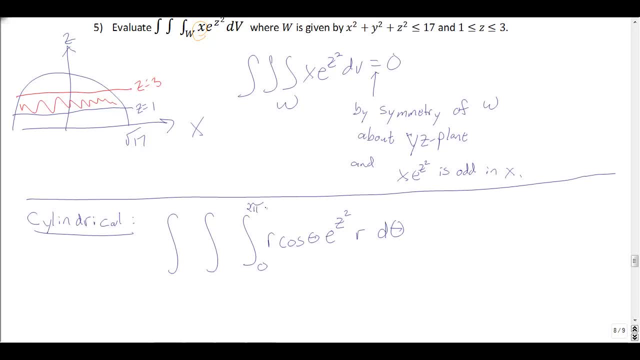 Theta is going to go zero to two pi here, and then what we want to do is we want to set up bounds for dz and dr. I'm going to do dz first and then dr. Now, one issue here when I think about the r is: if I'm sort of out, let's just sort of draw this. there's some line down here. let me draw a straight line here. 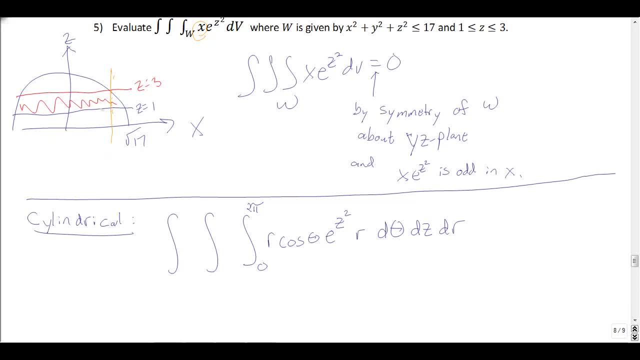 So if I'm to the left of this line with my r, z starts at one and goes to three, But if I'm to the right of this line, z starts at one and goes to this sphere equation. So that tells me I'm actually going to need two triple integrals to set this up. 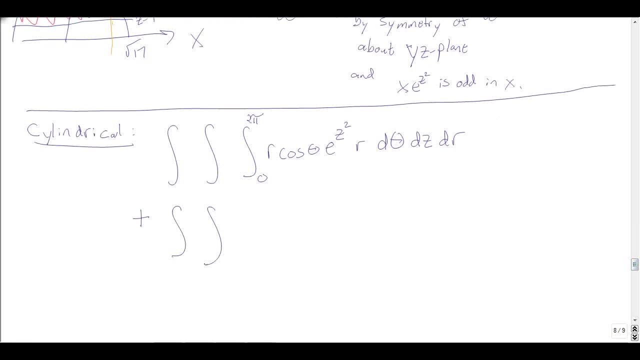 So I'm going to get one triple integral plus another triple integral. everything's the same so far. cosine theta e to the z squared r d theta, dz, dr. Let's look at the picture. Let's look at the picture. 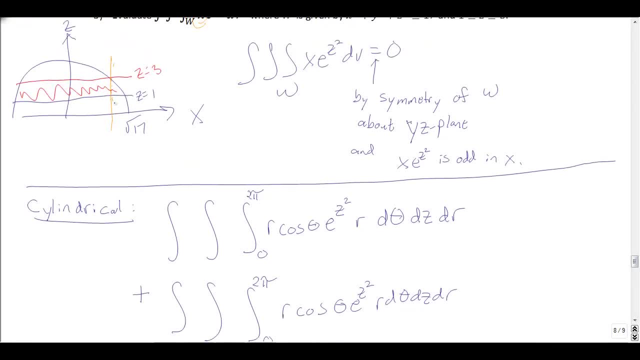 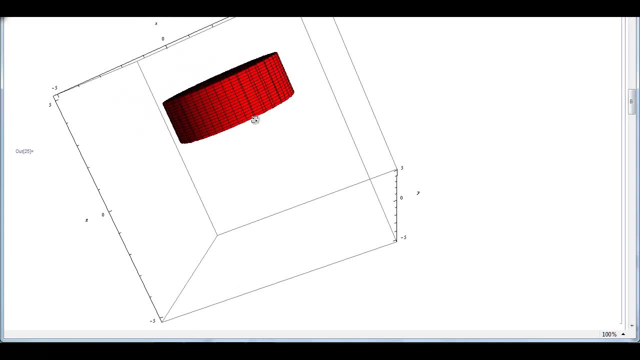 Let's look at the pictures of these two regions here just so we get a sense three-dimensionally of the two parts here. So when we go down, this is actually the region here where we have z going one to three, where that r went out to some point. 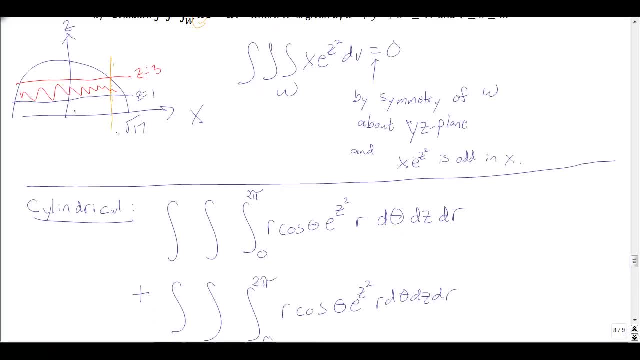 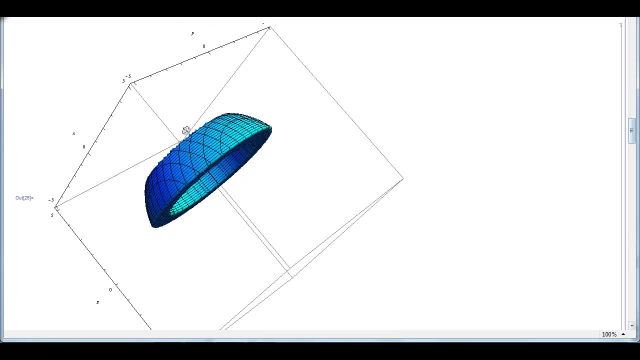 So that was on my graph. that was sort of this r to the left of this orange line, To the right of the orange line, a sort of accurate picture here. Mathematica looks like this here, So we get sort of a- well, sort of a- donut-looking thing, I guess, here. 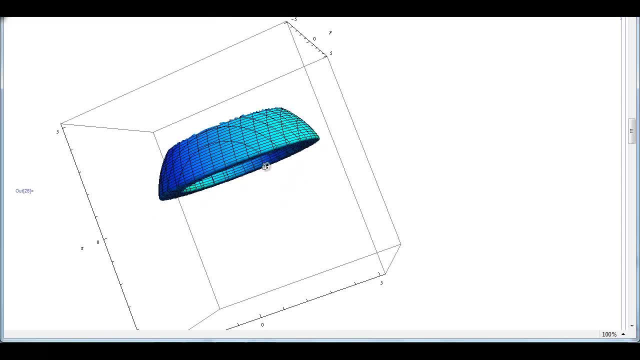 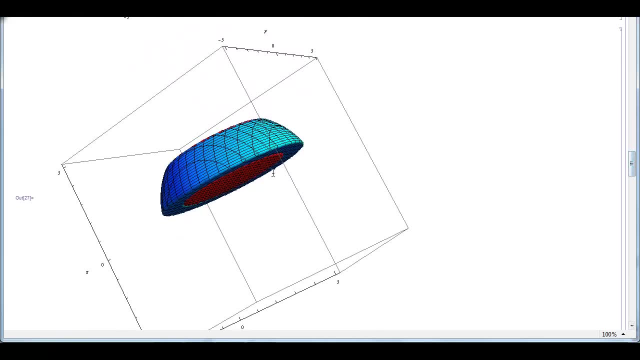 You've got this. on the bottom This is z equals one, But on the top I'm going to go to this sort of curved surface here And if I put those two together, here's sort of an image with those two together. 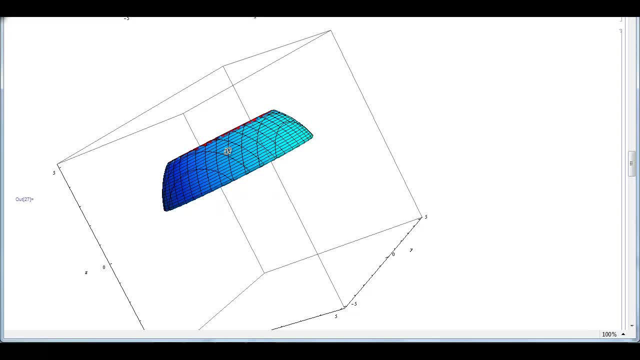 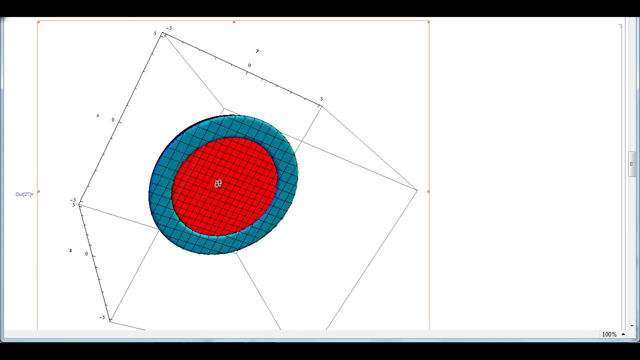 you can see sort of the first bit in the red, the second bit in kind of the blue there, And so you can see how those sort of nest here together And basically we're taking a cross-section whoops like this where here we go r equals zero to some point. 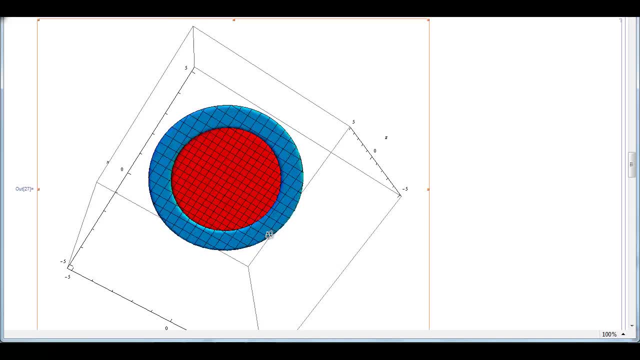 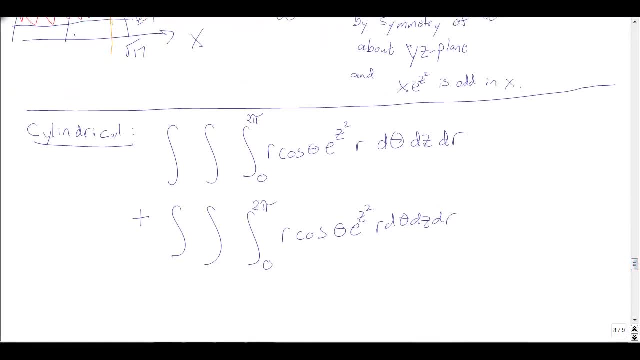 and then from that point out to sort of the final r. So those are our ranges. OK, So let's go set up our integral bounds, that in mind. So z the first one, let's do this. the left one, z went from one to three. 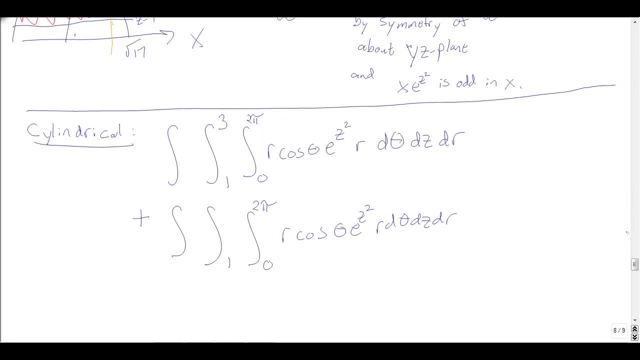 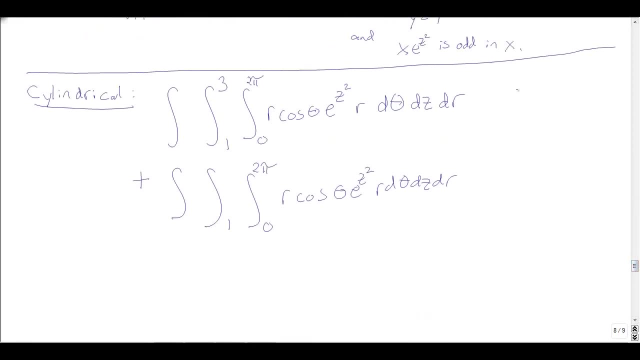 On the second one, z starts at one, but it goes to the sphere, sort of up to the sphere. Our sphere equation was- let me do this in another color- was x squared plus y squared plus z squared, well, equals 17.. 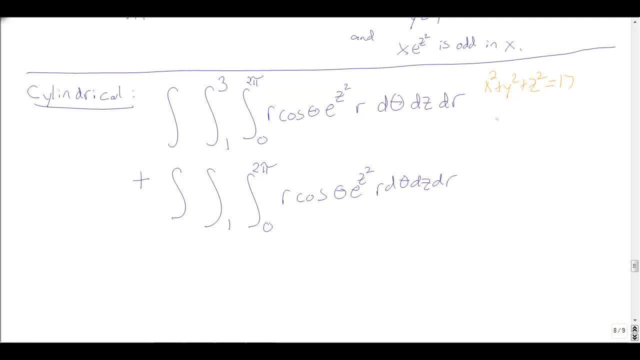 17 on the sphere, less than or equal to 17 would be the ball here. x squared plus y squared is r squared in cylindrical, And so z squared is 17 minus r squared. So z would be plus or minus the square root of 17 minus r squared. 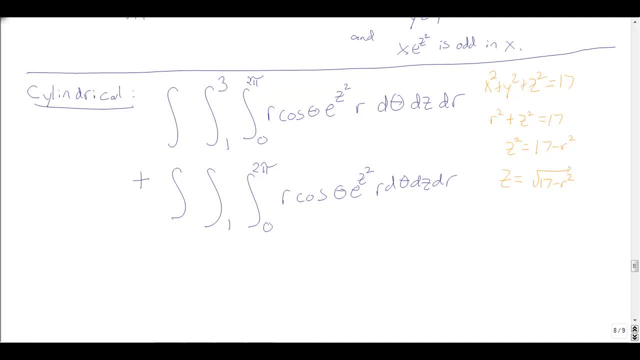 But we know we're having z from one to three, so z is the positive square root. So this upper bound is 17,. square root: 17 minus r squared. OK, And now. OK, The r bounds. well, so what we need to do is the first integral again is going to get. 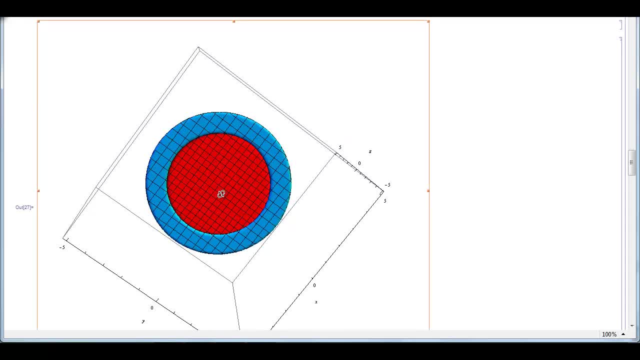 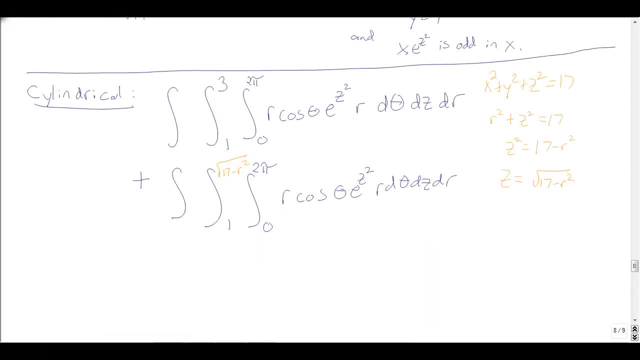 sort of the r bounds of this red circle if we rotate this up And the second integral is going to get sort of this blue kind of ring on the outside. So the red circle, well, that's when we think about it in our drawing. that's sort of right. 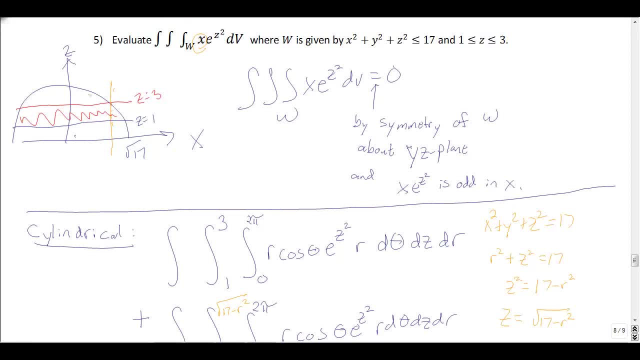 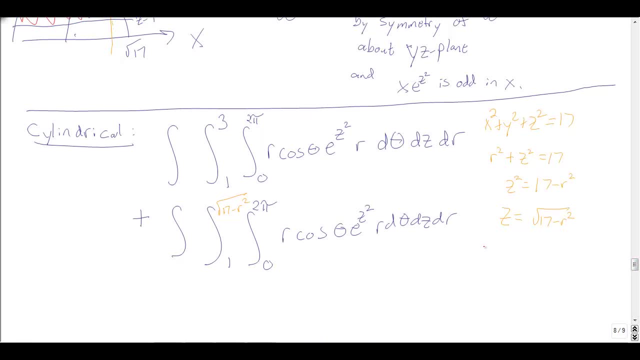 here, So that's z equals three where that intersects the sphere. So what we get is our sphere equation is r squared plus z squared, So that's z equals 17,. but we know z is three when we intersect that sort of plane. 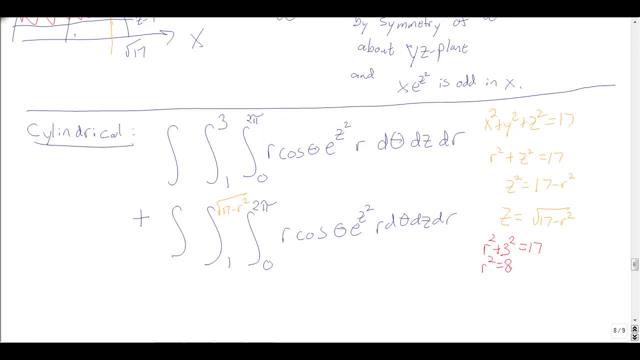 And so we get r squared equals 17 minus nine, that's eight. So r is square root of eight plus or minus, but we know it's a positive r. So what we're going to do is this sort of first one. we're going from one to three. 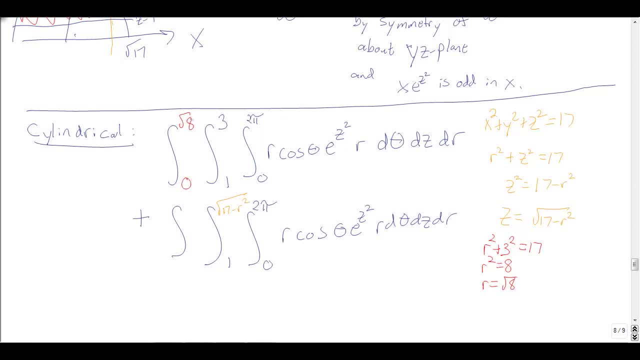 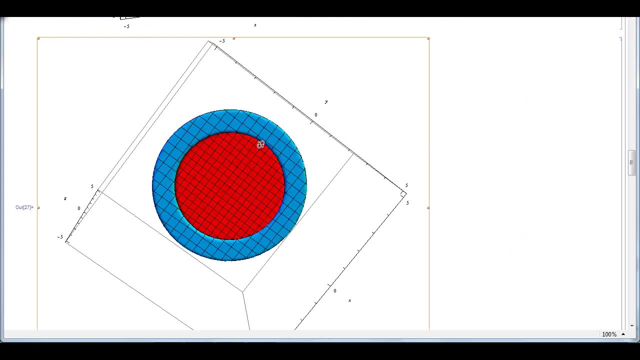 we can start r at zero and we end up at square root of eight. Now the second integral starts at that square root of eight And then it goes out. so it's sort of the same square root of eight and it goes out. 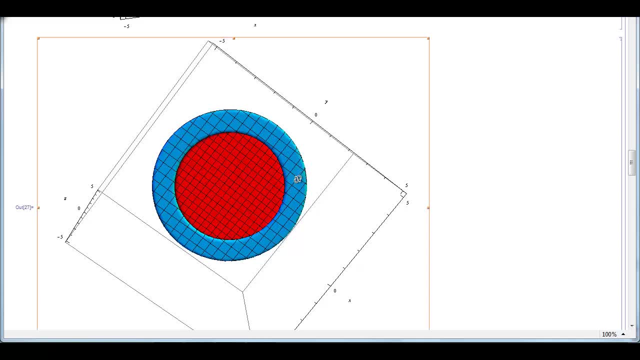 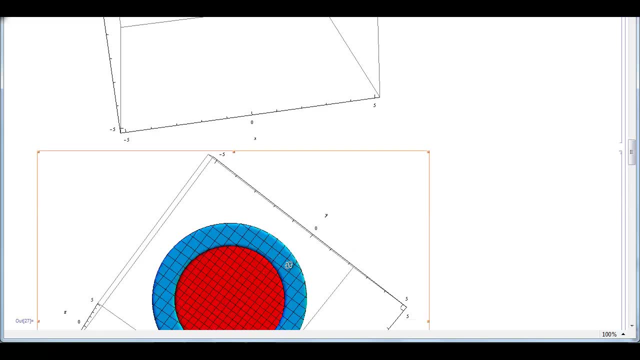 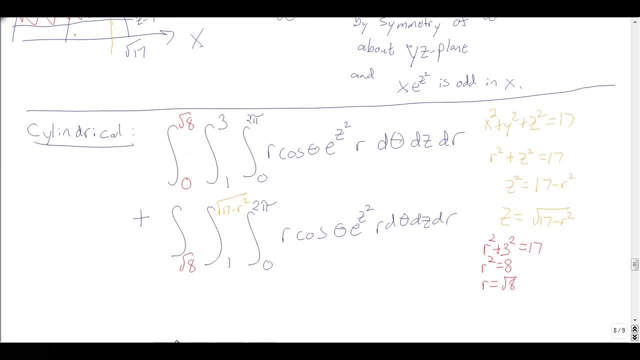 to this outer ridge here. Now that outer ridge is the sphere, rotate this down. it's not really going here. oops, there we go. Rotate this down so that outer ridge is the sphere when z equals one there. So what we can do is sort of the same kind of trick here. 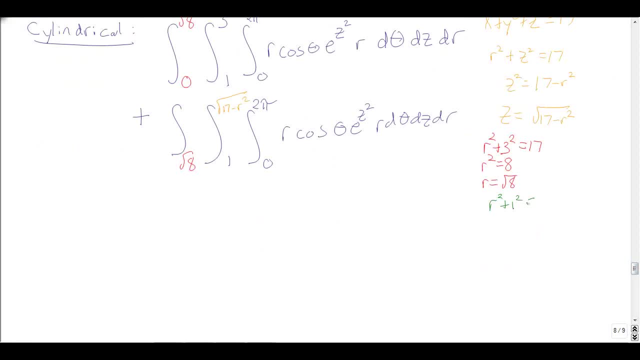 We can plug in: r squared plus one squared equals 17.. So r equals 17.. 17 minus one r squared equals 17 minus one. r squared equals 16, that gives me an r is four. So I go from square root of eight out to four. 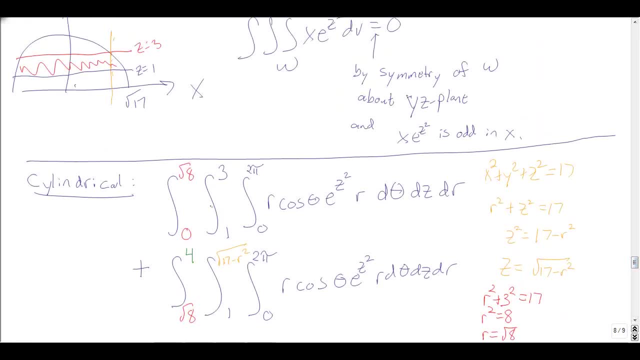 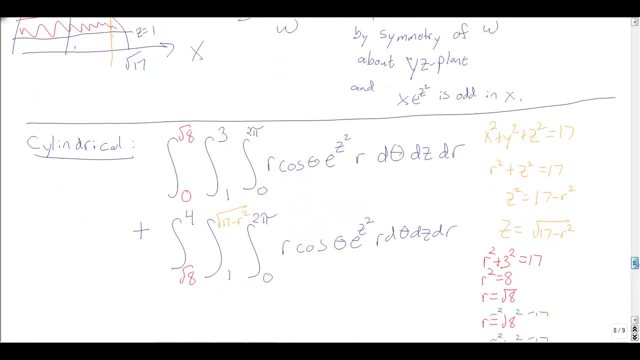 And there you have sort of set up in cylindrical coordinates here to be able to evaluate this integral. So let's go through and actually do the evaluation now. This is going to go really nicely. I'll say right away: I look at this and I'm worried about this. e to the z squared. 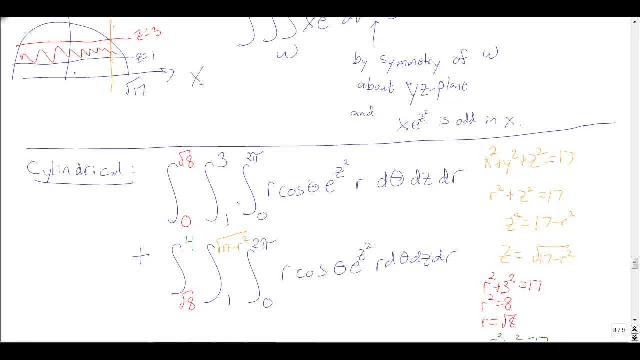 So I don't know how to integrate e to the z squared. In this first integral in particular There's bounds. I mean we're integrating over a cylinder. effectively that red cylinder from the Mathematica drawing here means all my bounds are constants. 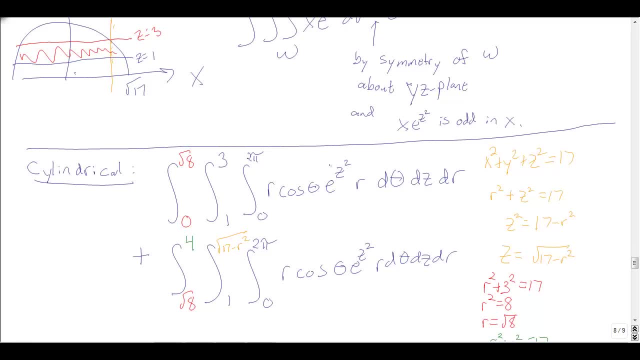 There's no variables, so I'm not going to get a z to pop up in some integration. So I'm kind of worried about that. Something nice is going to happen, though. Second one: still there's no z's in my bounds. I have an r but no z's. 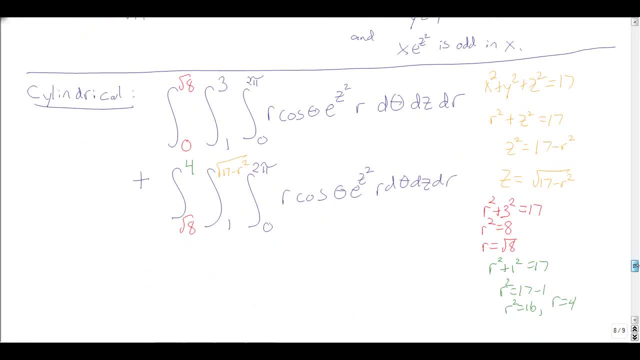 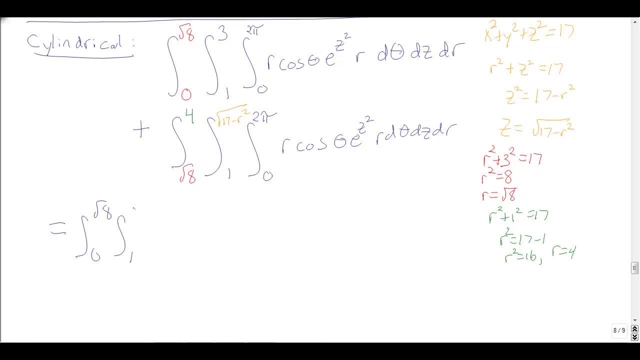 So I'm worried about integrating e to the z squared. So this is where I'm going to rely on doing theta first. So I'm going to get my first integral. so zero to square root of eight, integral one to three. Okay, I get the stuff without theta. is r times r, that's r squared. I have an e to the z. 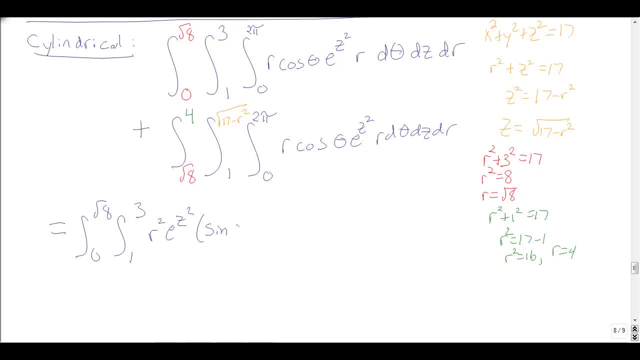 squared and then cosine, theta integrates to sine theta, and I do that evaluate from theta equals zero to theta equals two pi, and then we have a dz, dr, The second integral- I'm going to add this through. we get a square root of eight to. 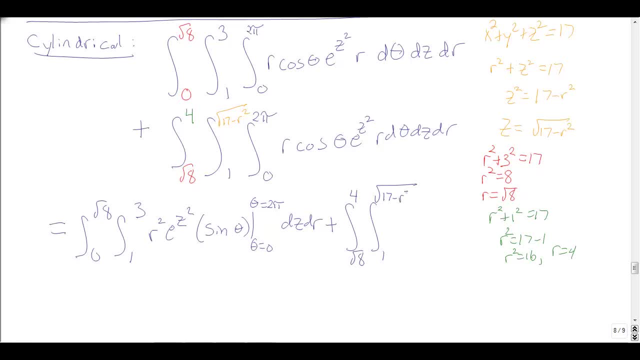 four one to square root, seventeen minus r squared, We get the same r squared, e to the z squared. I'm going to clear some space here- and I get times cosine. no, not times cosine. well, it would be cosine theta. but I want to integrate. 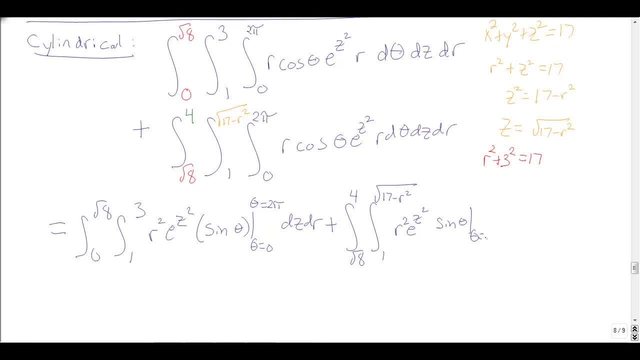 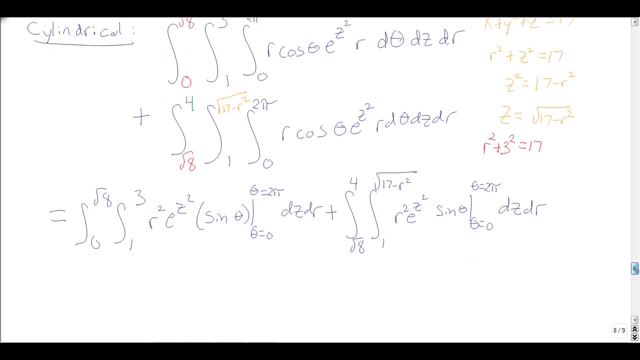 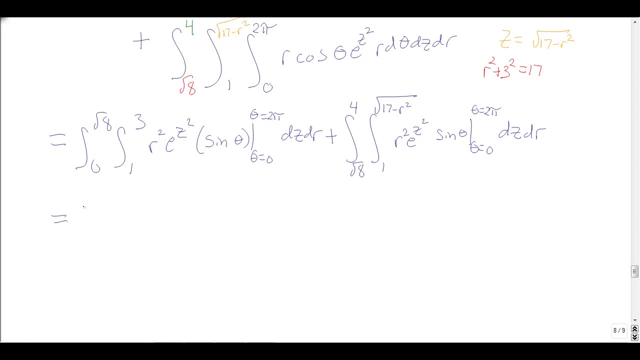 that and I get sine theta where I go from. theta equals zero to theta equals two pi, and again it's a dz dr integral. Okay, so now, when we evaluate this, well, sine of two pi is zero And sine of zero is zero. so you get zero to square root of eight, integral one to three. 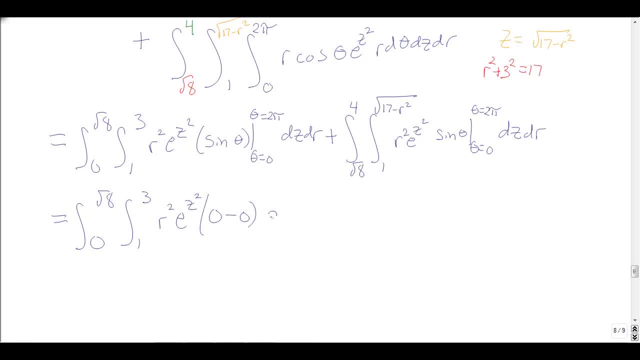 r squared e to the z squared. zero minus zero dz dr. Same thing with the second integral square root of eight to four. one to square root. seventeen minus r squared, I get r squared e to the z squared, I get sine of two pi is. 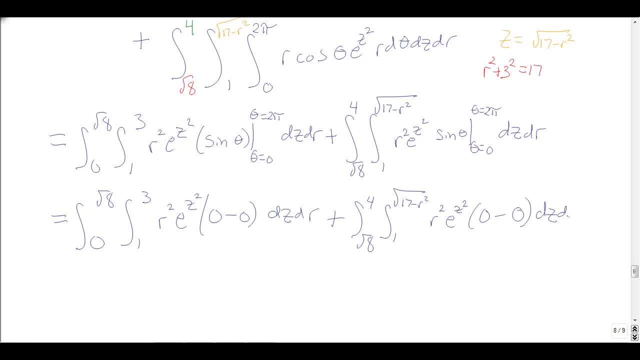 zero minus sine of zero is zero, dz dr. So now our integrand becomes zero, The function we're integrating becomes zero on both of these. so this whole thing ends up to be zero plus zero. that gives me a zero. Okay, so cylindrical coordinates. this works out not that bad. I mean it's a little bit. 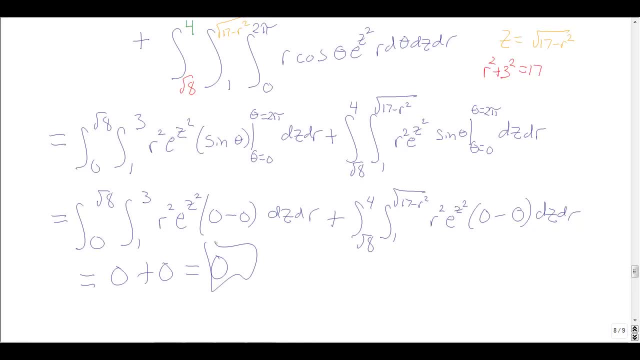 tricky. you have to split it into two integrals. do some work. none of the integration is hard the way we did this. note: if you tried to put that d theta on the outside and integrate with dz first, you're going to run into trouble because you're going to have to integrate. 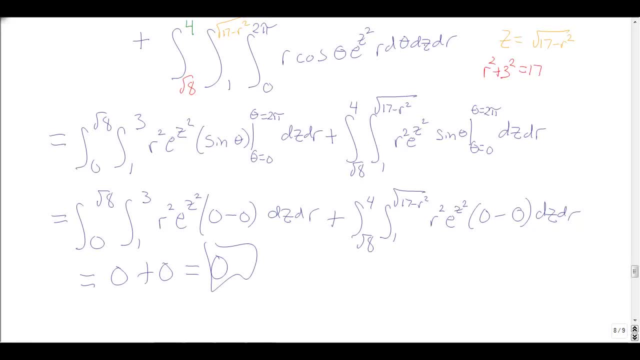 e to the z squared, which does not have a sort of nice antiderivative. So the theta on the inside is really the way to go. a lot of times you can do that with the trig function. sometimes they'll give you a zero and it'll save you work and 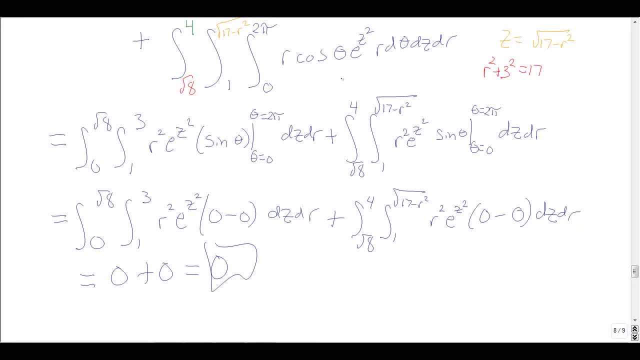 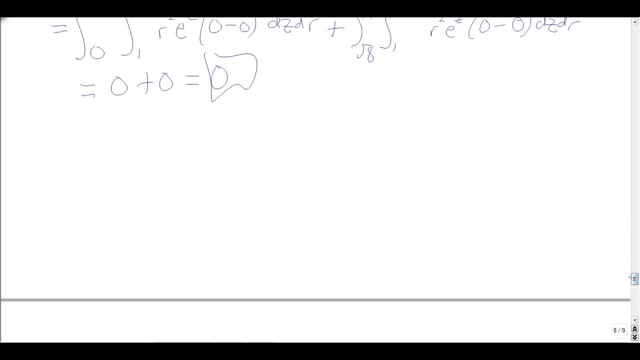 that's even if you didn't pick up on the symmetry of the problem right away, But symmetry is probably the way to go, really. Okay, let's do this in spherical as well. Let's do this in spherical. so what we're going to get here? let's maybe just go redraw. 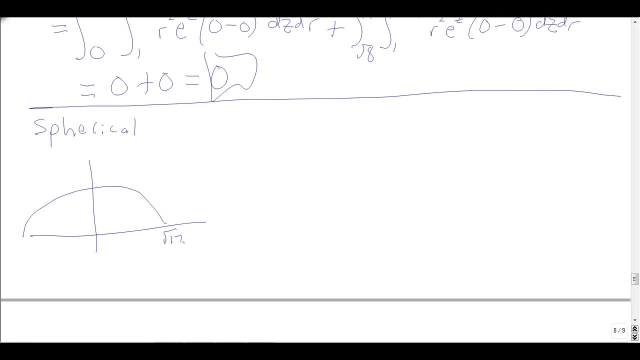 our picture. So we have a sphere of radius, square root, 17,. this is the sort of xz, and then I chop this with planes: z equals 3, and then there's another one at z equals 1.. So in spherical, what we're going to do is we're going to think about: okay, start out. 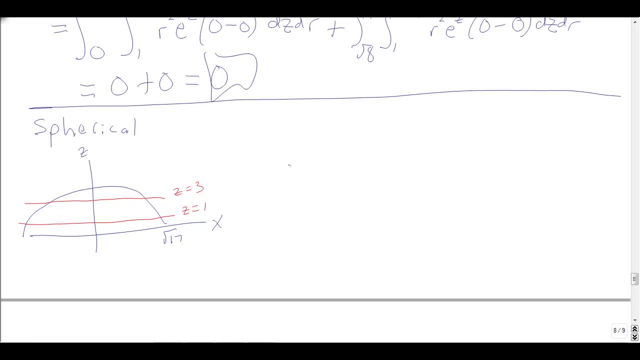 sort of at for rho. so let's maybe- well, let's- set up the spherical, so let's just do this as spherical. We have an x, So the function we're getting is x, e to the z squared, So the x is rho. that's going to be a cosine theta, but generally write this as rho sine. 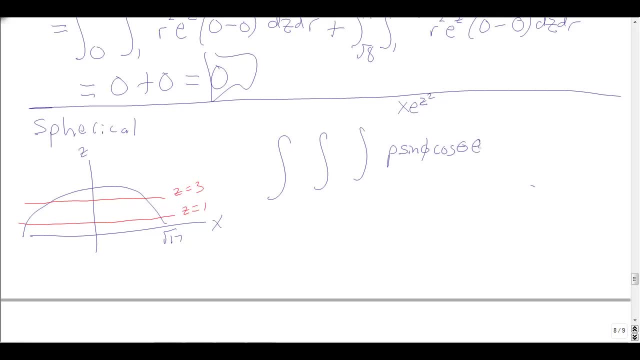 phi cosine. theta e to the z. z is rho cosine phi squared, and then my Jacobian is rho squared sine phi, And I have to set up an order of integration. Again, I'm going to use the same trick with cylindrical. I'm going to do theta first. 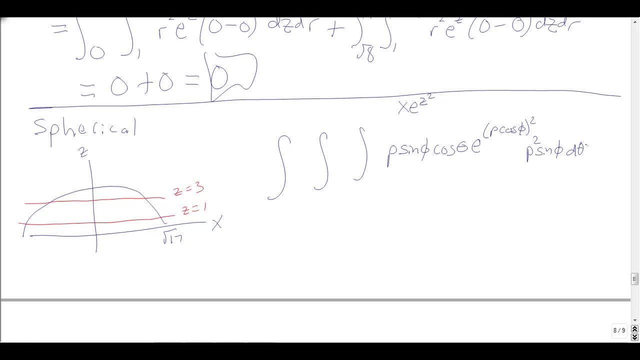 and then I'm going to hope. I hope that that gives me an integral of zero and I don't have to really worry about the others, but we can set up bounds anyway. Then I'm going to do d rho, d phi, whoops, d rho and then d phi. those are my bounds. 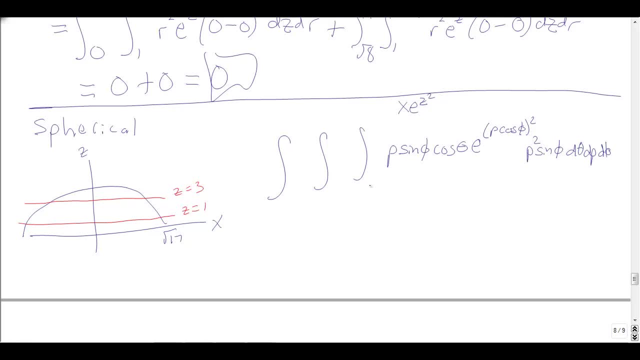 What I'm going to get then. okay, theta, I rotate all the way around. theta goes zero to two pi. Now you can look at this and see the only theta here is the cosine theta. so I'm going to integrate cosine theta from zero to two pi. 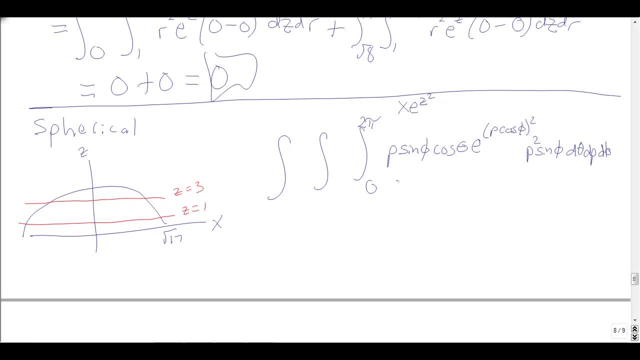 That's going to give me zero. So I look at this right here and say, well, this is zero. you're going to have to split this up into two triple integrals. each of them will be zero. Here I don't really care what the bounds are, so you don't technically need to do this. 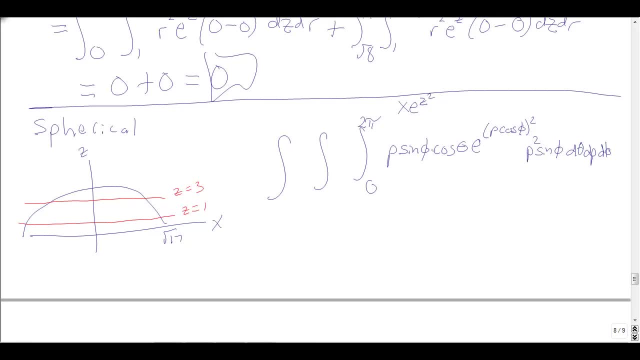 but the point is, how do I set up the bounds for the shape? what if I had a more complicated thing and I didn't have that cosine: theta. Okay, so that's theta. now phi and rho. well, let's look at rho here. 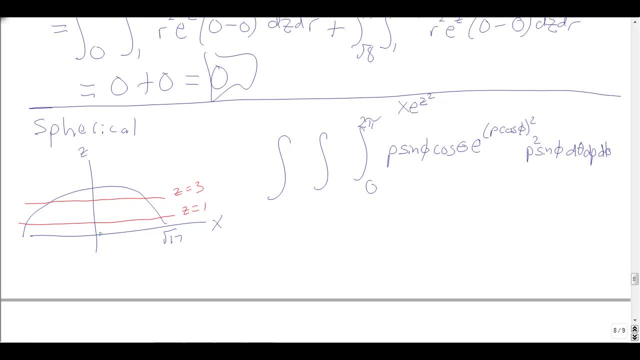 So rho is going to start at the origin. so let's just take a sort of ray out here. So here it's going to start at the origin. it's going to go at this point. it's sort of get into my surface, so that's at some point there. we had to find an equation for. 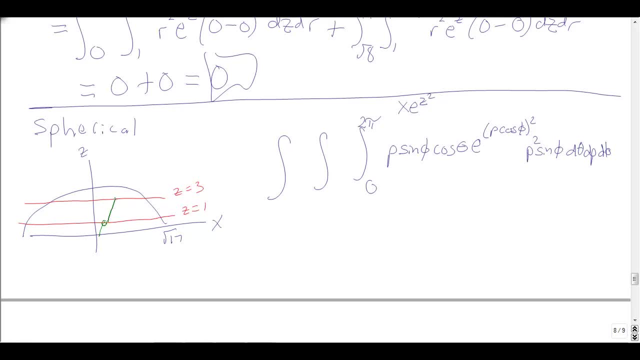 z equals one, and then I go out and I sort of leave the surface at z equals three. So we're going to have to come up with equations in terms of for rho and phi, for z equals one and z equals three. but if I go and let's say, let's do an orange if I shoot out over, 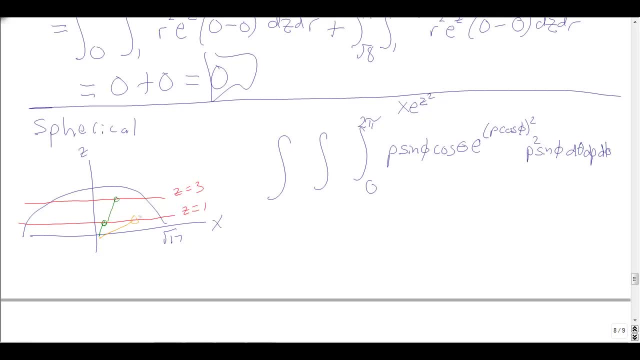 here I'm going to hit that z equals one, But then I continue. on the surface I sort of end or out of my solid on the sphere. So I'm going to end up with two different triple integrals and these are going to split. 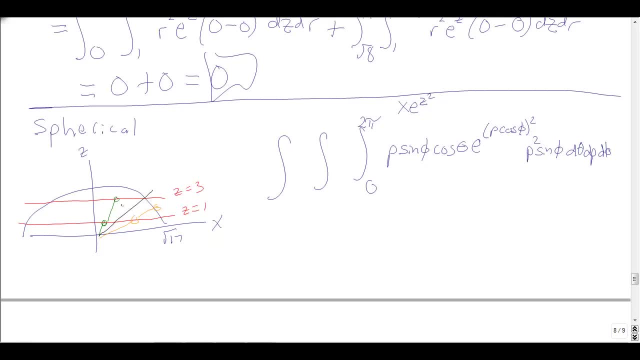 on sort of this ray here. So I'm going to get sort of this wedge shaped thing. I'm going to draw this here too, sort of this wedge shaped thing inside as one integral, and then I'm going to get sort of this part: 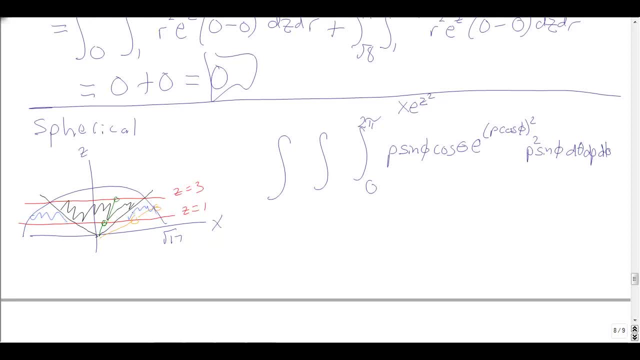 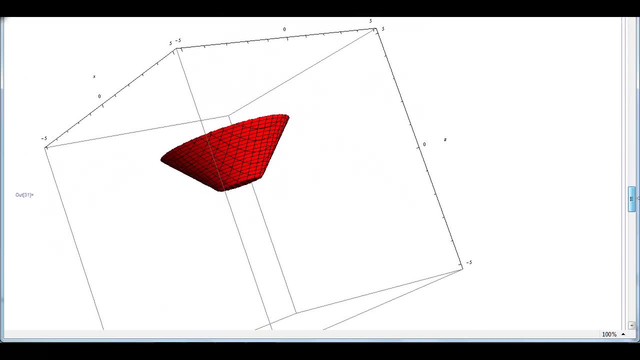 with this part rotated around for the other triple integral. So you've got my ugly drawing to look at. let's look at Mathematica as well. So that wedge shaped thing. here's what that is. So this is the black rotated around. you're going to get this part here and you can see. 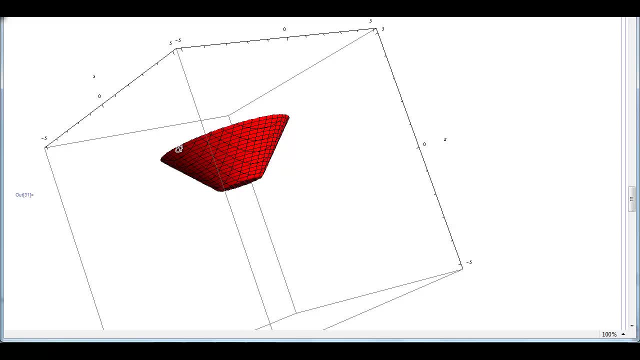 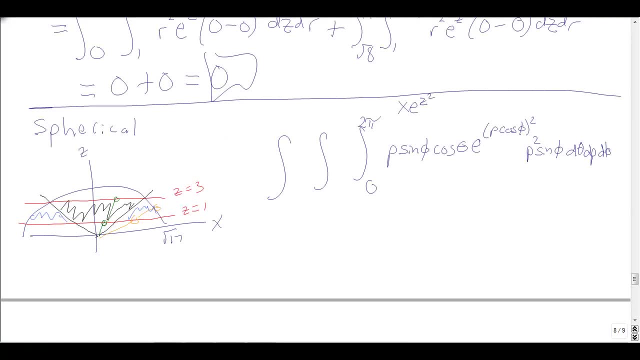 rho goes through the bottom, that's at z equals one, and it goes out to the top at z equals three. Now the sort of blue shaded part here rotated around so it kind of looks almost like a triangle, but this side is curved. 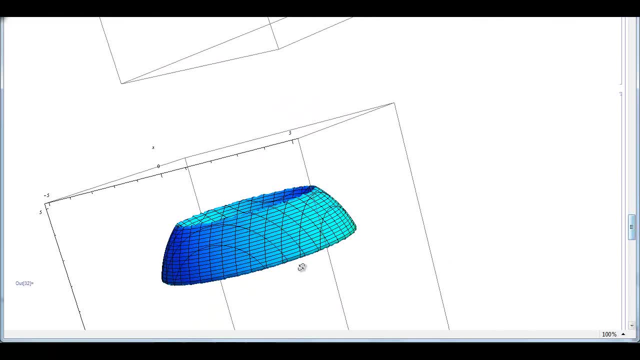 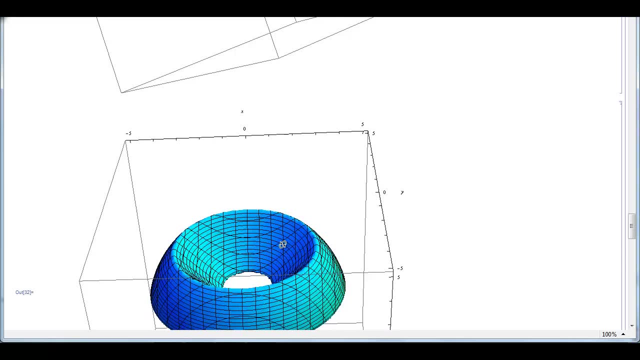 What that's going to look like. Is this going to look like this? This guy here, so we rotate this in and you can see it's sort of well, the rest where that red sort of plug would fit in here, kind of a thing. 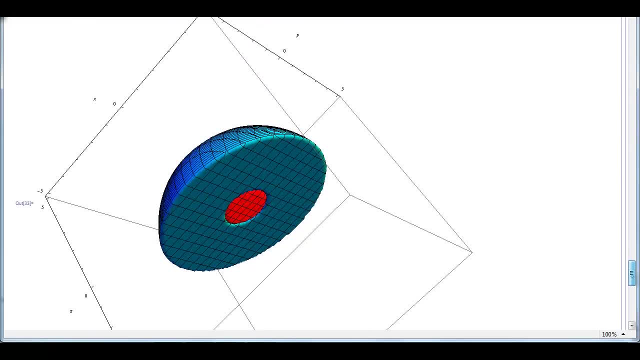 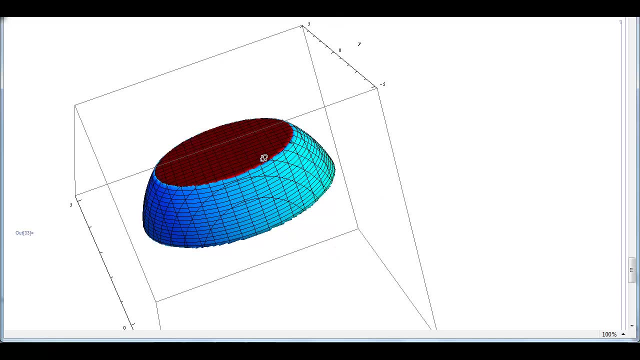 So it's that rotated around, and when you put them together sometimes it helps to see what's going on here. what we've got is this shape. here you can see the top: z equals three. so that's where the red- I start at z- equals one in both. in the red I end up at z equals. 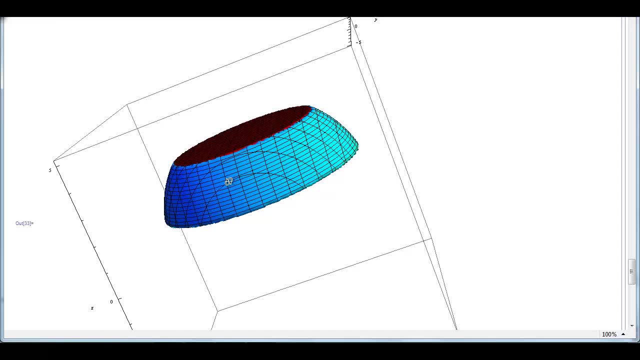 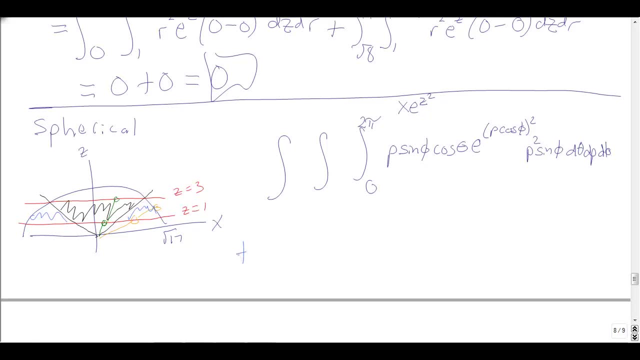 three in the blue sort of the ray from the origin goes out and hits on this here. Those are sort of the visuals of what's going on. So what we're going to do is set up a second triple integral. we're going to get a zero. 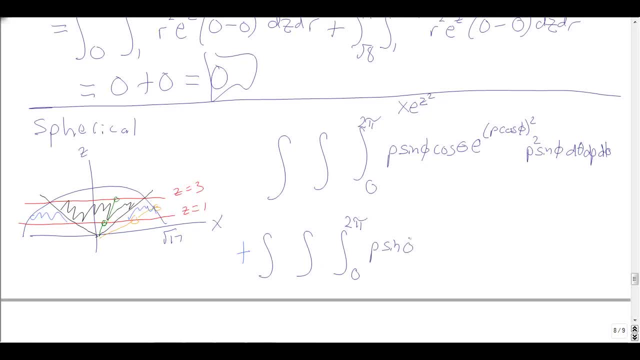 to two: pi rho sine phi, cosine theta. we have e to the rho cos phi squared. then I get my rho squared sine phi and I'm going to do this: d theta, d rho d phi. So that's really That's really sort of our two integrals here. but now we need to do bounds rho. well, let's. 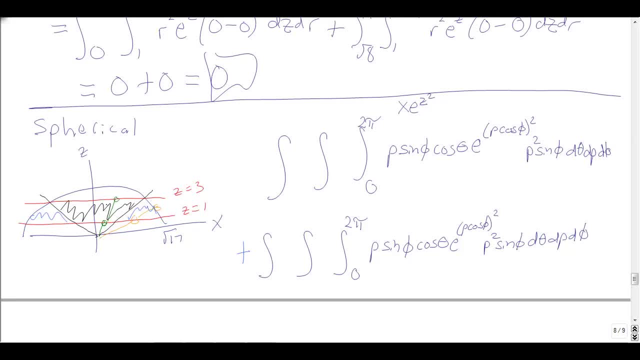 think about phi first. phi might be easier. So, on this black region, phi's going to start at zero, starts at zero and it's going to go out to whatever this angle is here. So on that angle, let's see if we can figure out what that is. what you could do is draw. 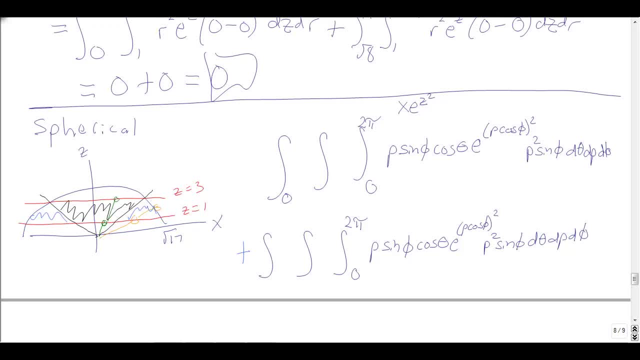 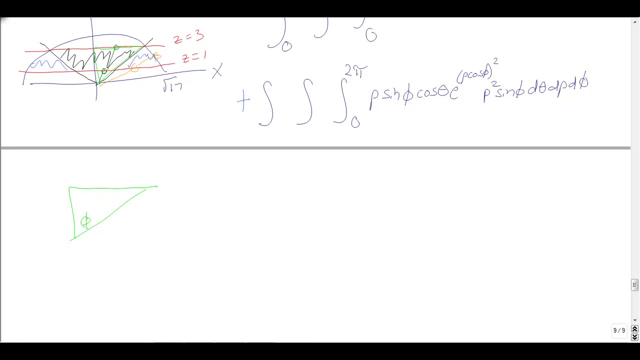 a triangle. so let's see here, try to do this in sort of a bright green. I have a triangle sort of right here. so that triangle, what I'm going to get, triangle like that. there's my phi, this top. well, I'm at, z equals three. so that leg is three and the hypotenuse. 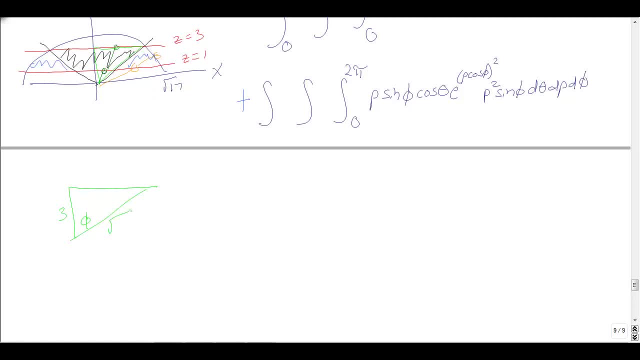 that's part of that sphere of radius, square root of 17,. so that's a square root of 17.. And so what I'm going to get here's that top is inverse cosine of three over square root of 17.. So kind of an ugly. 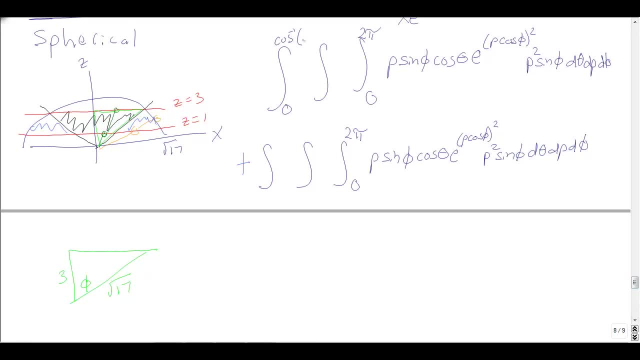 bound, but it's cosine inverse 3 over square root 17. so that's what we've got. the other bound. I'm gonna start at that cosine inverse 3 over square root 17 and then I'm gonna have to do a different triangle to find sort of the angle when. 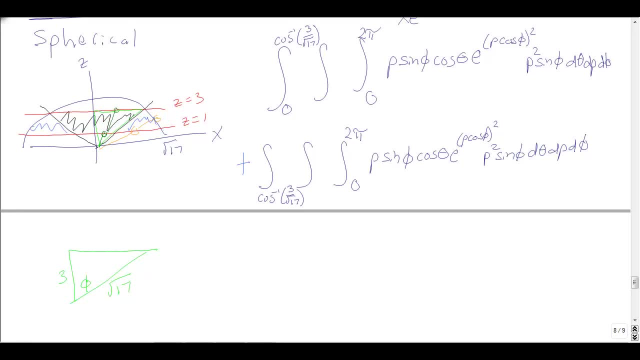 Z equals 1, so that triangle. let me do a darker green here, so I'm gonna have one side here, one side out here in my hypotenuse there. so that's gonna be a triangle like this here. here's really the Phi that I care about. that should be. 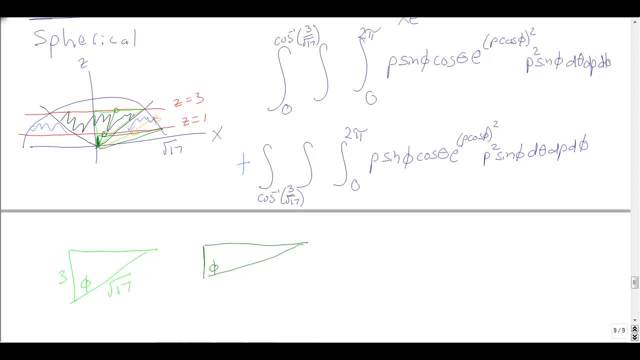 something slightly less than PI over 2. this leg is going to be 1 because that plane is Z equals 1 and again the hypotenuse is square root 17, so we get a Phi being another inverse cosine. so cosine inverse of 1 over. 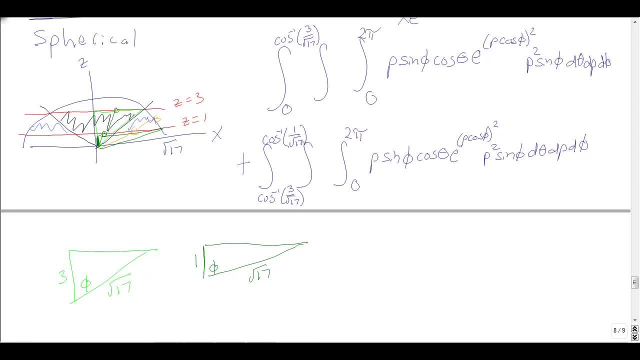 7. so we get a two and two equal sign, and alright. so we get a three and a two and two equal sign, and alright. so we get a three and a three and a square root 17.. So there's our phi bounds. Now our rho bounds, so the first one up here we're going. 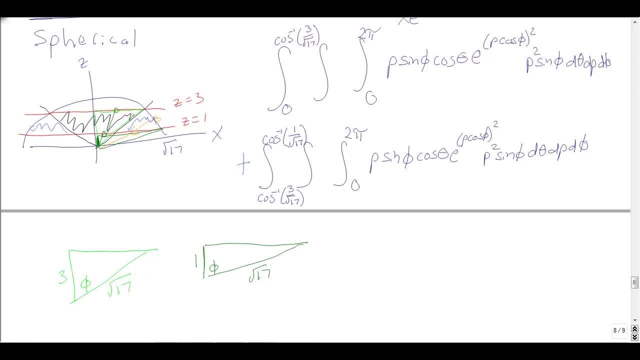 from z equals 1 to z equals 3.. So we've got to write those down: z equals 1, that's rho, cosine phi equals 1, and that tells me rho is 1 over cosine phi. So that was the starting rho bound. 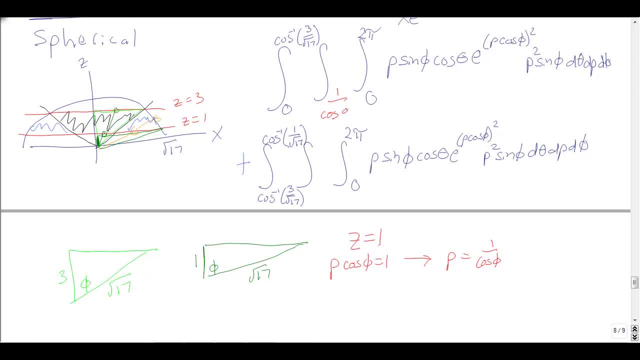 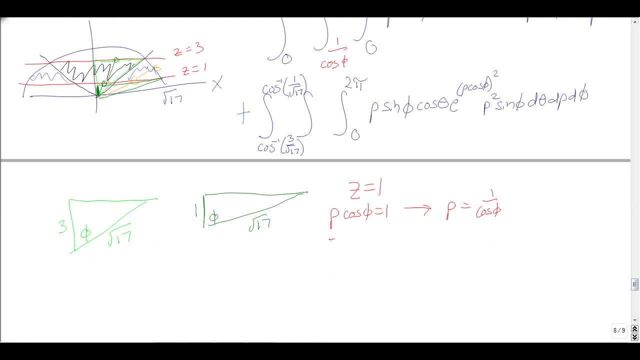 for the first integral, You get a 1 over cosine phi. The ending bound is the same thing, but I put a 3 where this z is. So what I get here is I get a z equals 3, and then rho, cosine phi equals. 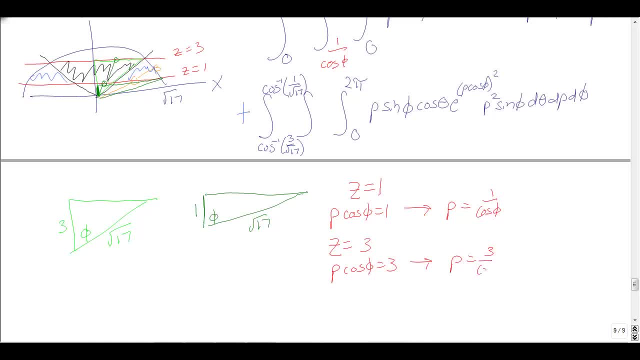 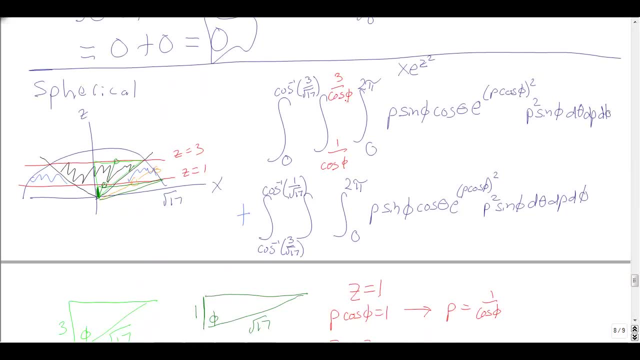 3, and so I get rho equals 3 over cosine phi. So my upper bound is 3 over cosine phi. Okay, the other one I'm going to start at on this sort of orange segment. here I hit the plane at z equals 1.. That's still the 1 over. 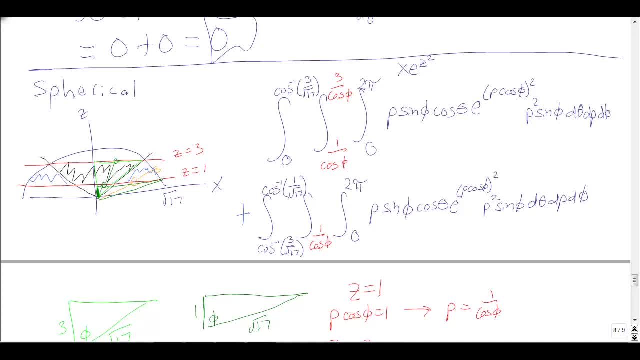 cosine phi and I go out till I hit the sphere. Well, the sphere is going to have radius, square root of 17.. So I pick up a square root of 17.. So there really is my big triple integral. Well, two triple integrals I have to do. Looks kind of intimidating, but again, when we integrate with 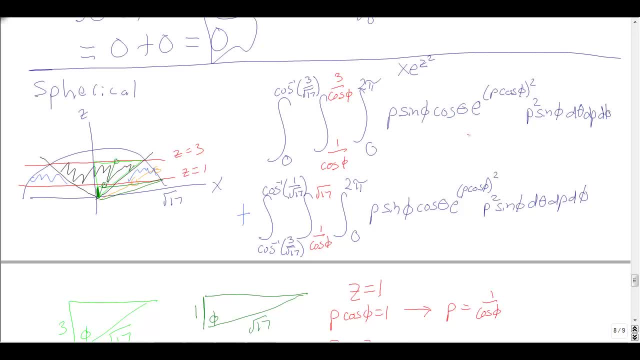 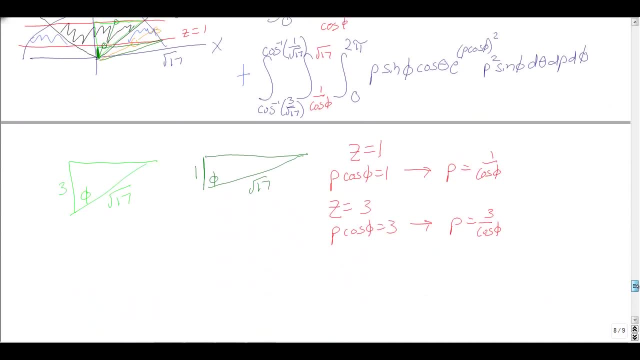 respect to theta. we get a cosine theta That's going to give us 0. So let's just run through that quick here. Our first integral down here was where you have an integral from. let's see, I forget what it was. 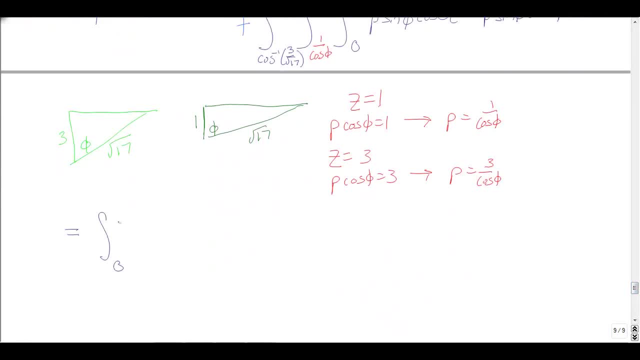 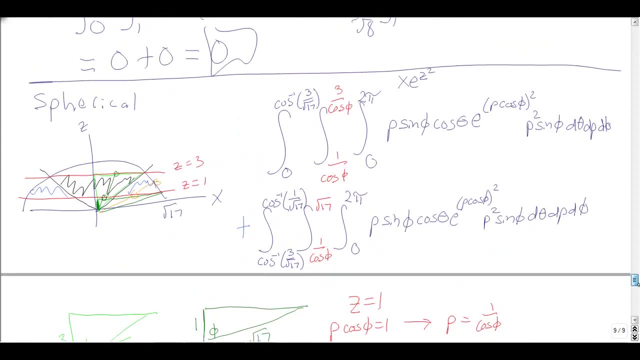 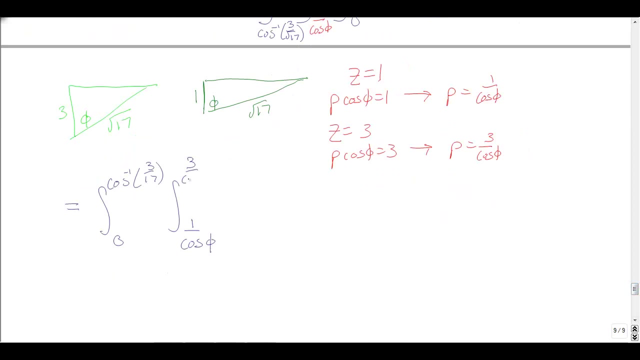 It was cosine 0 to cosine inverse, 3 over square root of 17.. The next bounds went from 1 over cosine phi to 3 over cosine phi, And then the thing I'm integrating. let's just simplify. it's going to be the same thing here I get. 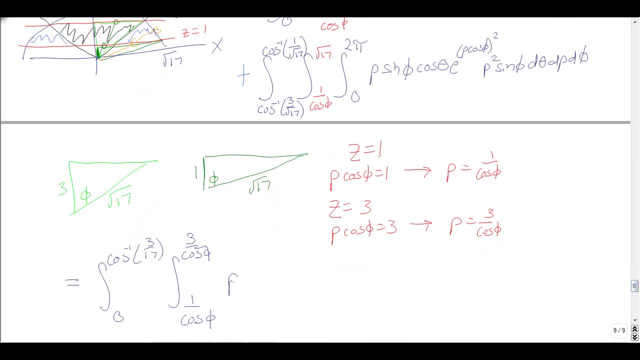 rho cubed. let me write this down: I get rho cubed sine phi times sine phi is sine squared phi. and then I get an e to the. it's going to be rho squared cosine squared phi. and then when I integrate cosine theta there, what I'm going to get is a sine theta I have. 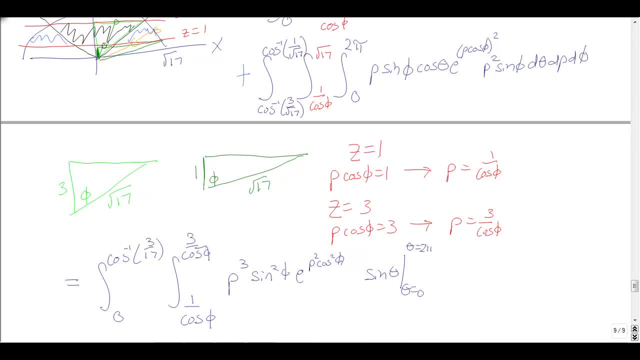 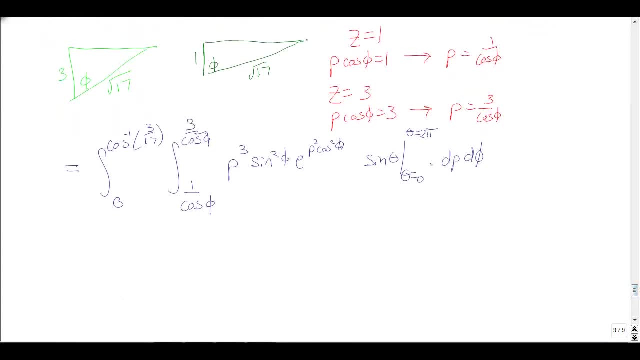 to integrate that from theta equals zero to theta equals two pi. and then I'm doing d rho d phi. so that's the first integral note. this part is going to give me a zero. so that whole thing, so this whole thing here, that whole thing goes to zero, and then we're going. 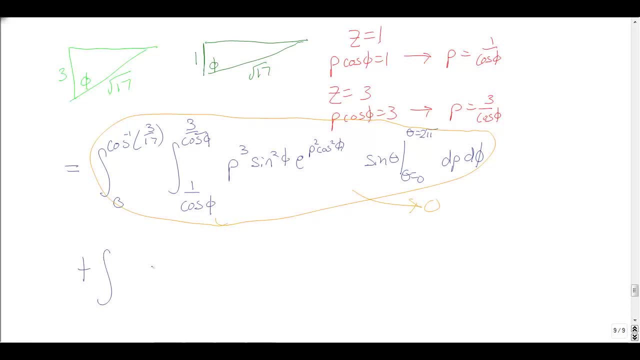 to add to it. let me write the plus down here, the second integral. the only thing that's different is these bounds, but that doesn't affect the fact that we get a zero here. so we're going to go from. this: was cosine inverse one over square root of seventeen. 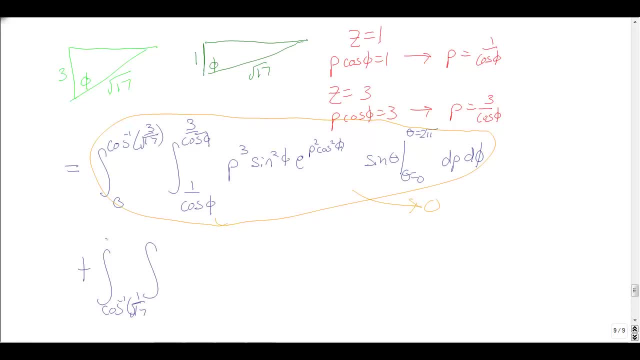 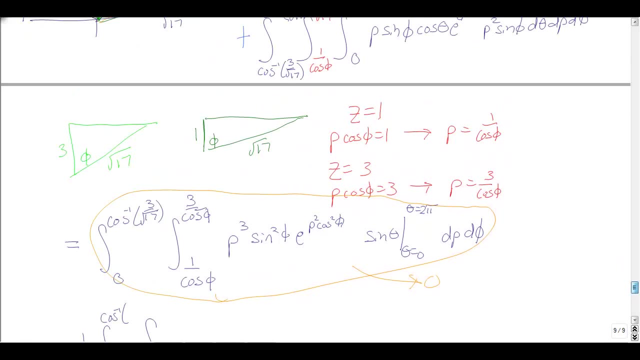 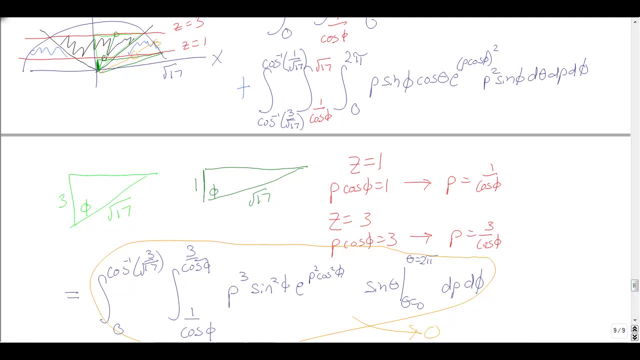 whoops, this was three over square root seventeen. I missed the square root in the first one, cosine inverse. to wait, no, let's go through this. one starts at cosine inverse. oh, I think I have the wrong bounds here. now I look at it so I started at z equals one. no, phi starts. 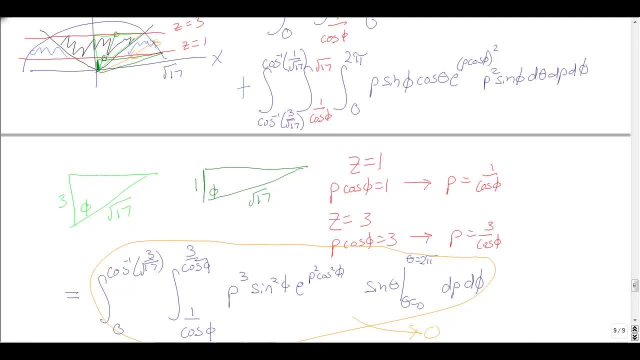 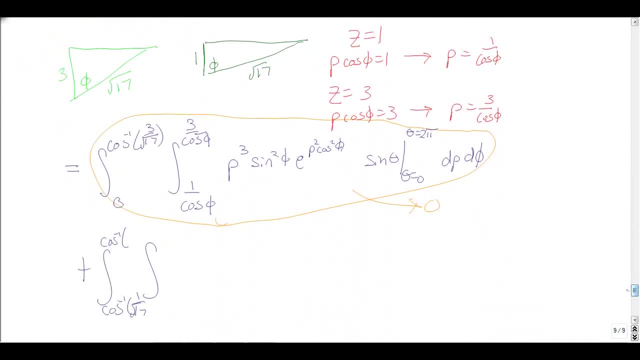 at cosine inverse three over square root of cosine inverse three over square root of seventeen, to cosine inverse one over square root of seventeen. that's good, Everything's good there. so I'm going to start at, but I start at, the bottom bound is the. 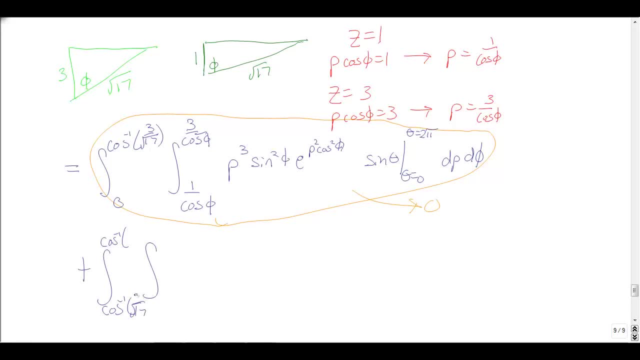 three. so this should be a three and this is one over square root of seventeen. I'm just going to make sure I have that correct. yep, okay, next bounds. I had a one over cosine phi and I went out to square root of seventeen, out to the sphere, and then I get this same.